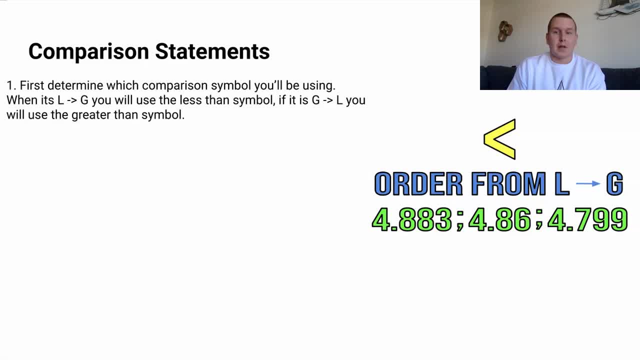 If it's greatest, greater to least, you will use the greater than symbol. So, since we're ordering from least to greatest, we're going to use the less than symbol. Remember, the less than symbol kind of looks like an L, and it does matter which way it's open towards. 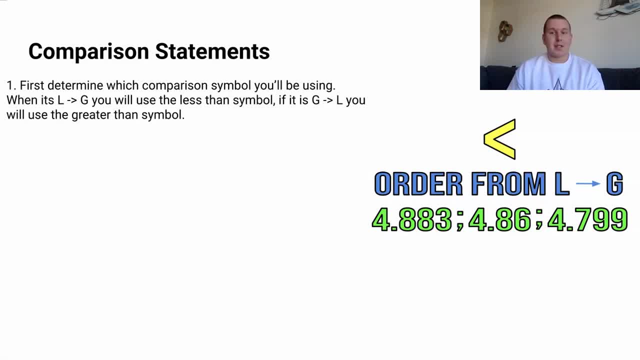 The way I remember this is, if it starts from least to greatest, I'm going to use the less than L's first, so less than. If it's greatest to least, then it starts with the G first, so I'll use the greater than symbol For step two. we're going to stack the numbers on top of each other. it does not. 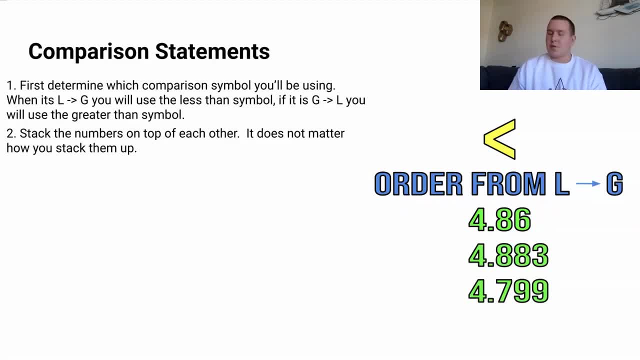 matter how you stack them up. So don't try to order the numbers right now. just put them in one straight line vertically, so we can compare them a little bit more easily. Step three: draw the lines between the place value to help more easily compare the numbers. This might seem a little familiar from the video we did the other day. 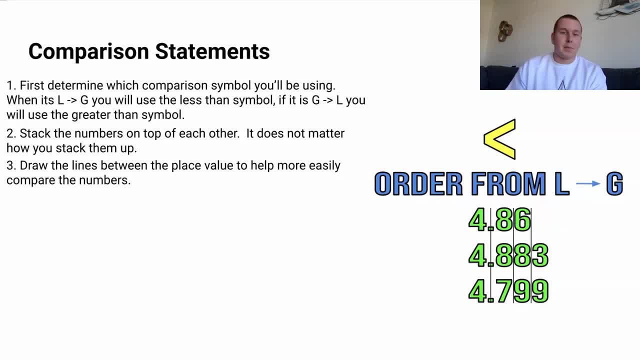 It's the exact same step. we're going to line them up, split them up and by place value. Step four: draw a zero in any of the blank spaces. Remember, when we add a zero to the right of a decimal, it does not add or take away any value. So four and eighty six hundredths is equivalent. 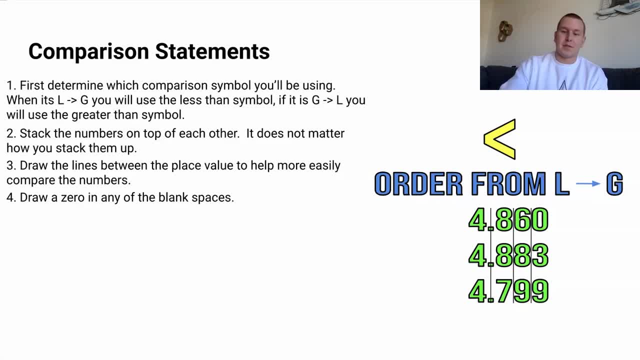 or has the same value as four and eight hundred sixty thousandths. Step five: this is the really important step. we're going to find the first number in the comparison statement. Once you find it, cross it out. Write that number first, followed by the symbol you'll be using for the. 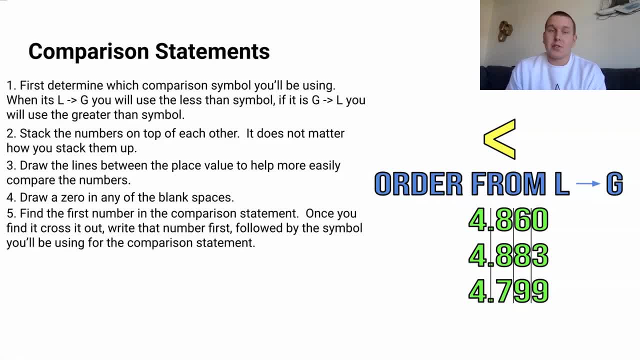 comparison statement. So we're ordering from least to greatest, so we're going to be looking for the number with the smallest value or the least value. So when we look at the ones place, all of them have four in it, so we can't really make a judgment there. We move over to the tenths place and it. 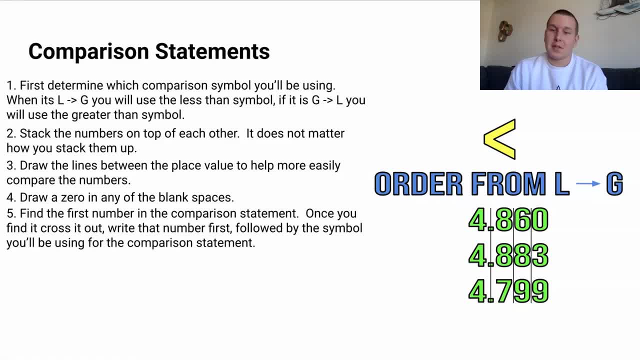 looks like that bottom number has a seven in it, which makes it smaller than the top two numbers. So what we're going to do is we're going to cross it out. I also like to put an l next to it, to know that that is the number that is the least, and then that number will start my comparison statement. 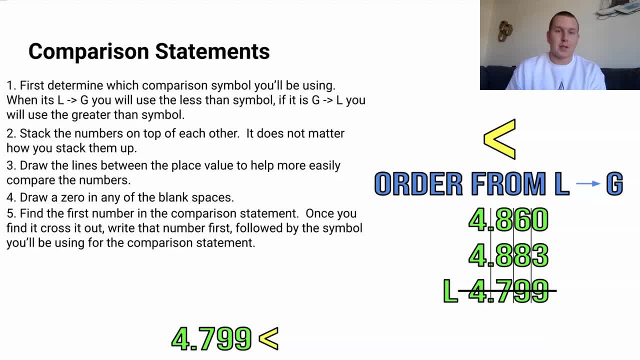 So we're going to use the less than symbol. We're going to continue to use the less than symbol when we're creating this comparison statement. Step six is: repeat step five until your comparison statement is complete. So we're going to go back through. We know the top two numbers are: 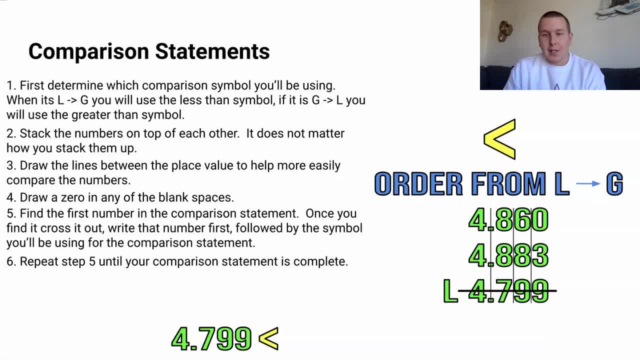 equivalent in the ones place and in the tenths place. So let's take a look in the hundreds place. It looks like six is less than eight. So our top number is going to be the next number that comes in our comparison statement. So we're going to cross out that number. put a g by the middle number. 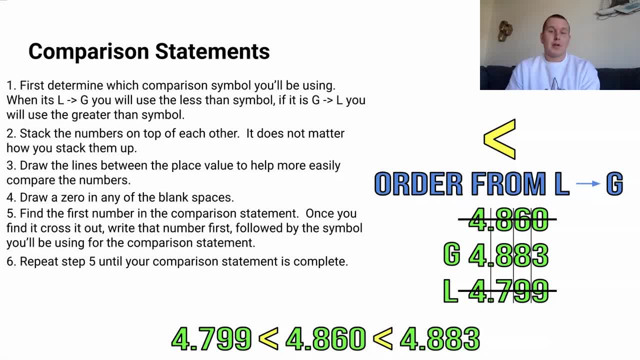 is the greatest, and then can our finish creating our comparison statement. Then our final step is to read your comparison statement out loud and see if it makes sense. So I would say: four and seven hundred ninety nine thousandths is less than four and eight hundred sixty thousandths is less than. 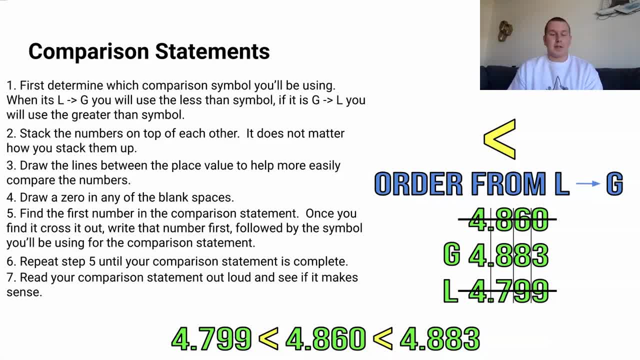 four and eight hundred eighty three thousandths, and that looks like it makes sense. It looks like we ordered it all up and it's all good to go. Now. one thing you may notice is that I kept the zero when I created my comparison statement. You could leave that out. You could have left it. 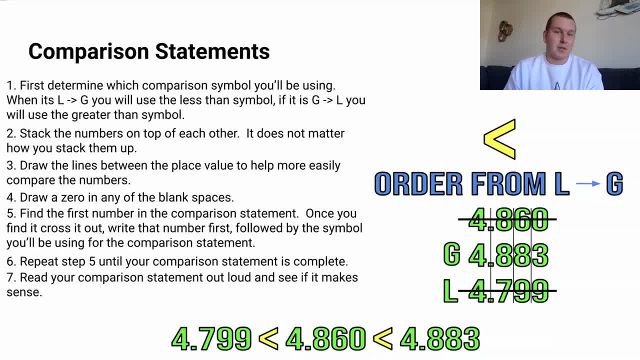 four and eighty six hundredths, but I like to include it just so it's a little bit easier to compare. So ordering numbers from least to greatest and greatest to least isn't too much different than what we did when we were just comparing two numbers, but there are a couple of slight differences. Let's 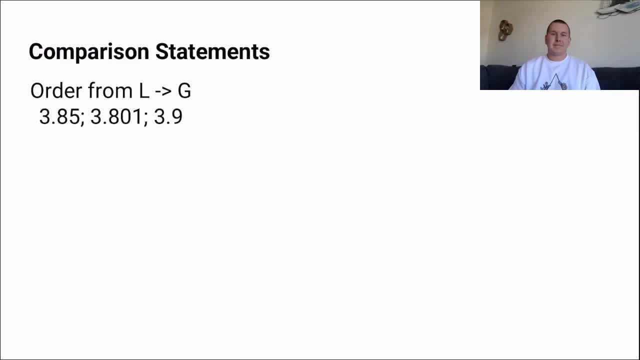 go ahead and practice a couple problems together, All right. so in this first problem, we're once again going to be ordering from least to greatest, So we need to figure out the symbol we're going to be using. Since it's least to greatest we're going to go the less than symbol. Remember it starts with. 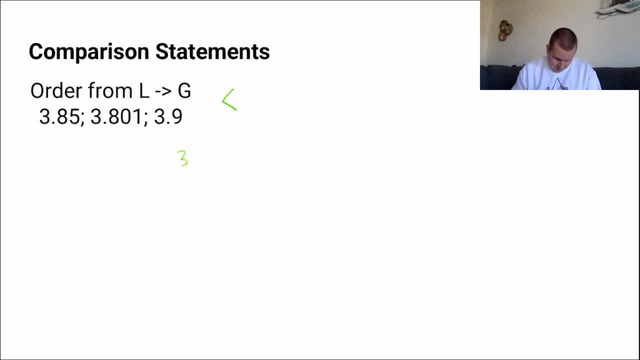 a symbol. So we're going to now stack these numbers up. It does not matter the order in which you stack them up. I'm just kind of going from left to right here And then, once we've stacked these numbers up, we're going to draw some lines in between them. This helps us more easily. 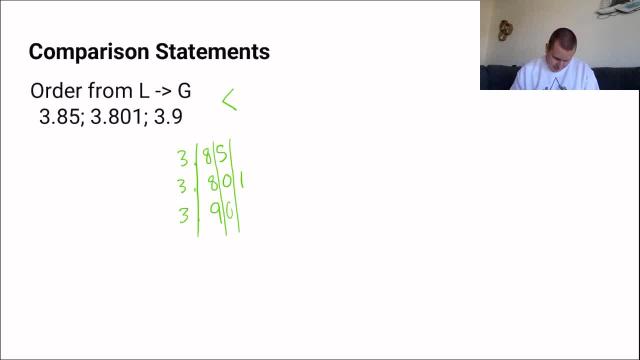 compare the numbers. Now, any place that there's a blank space, we're going to add a zero Again. that helps us more easily compare the numbers. Then we're going to go through and we're looking for the smallest number And the ones place. they're all threes And the tenths place. 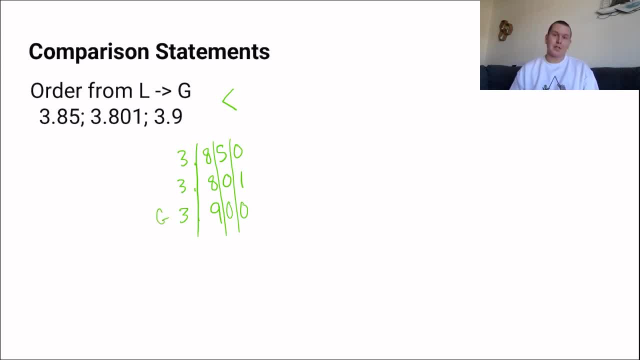 one of them is a nine, So I know that number is actually the greatest. So it'll be the last number in our comparison statement. We can kind of cross that number out now, since we don't need to use it. Then we go to the hundreds place And again we're looking for the smallest number And it looks like. 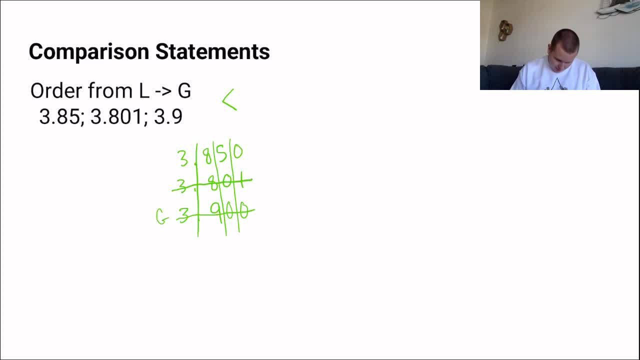 zero is less than five. So we're going to cross that out and that's going to be our least. So we're going to say 3 and 801 thousandths is less than The middle number would be 3 and 85 hundredths. 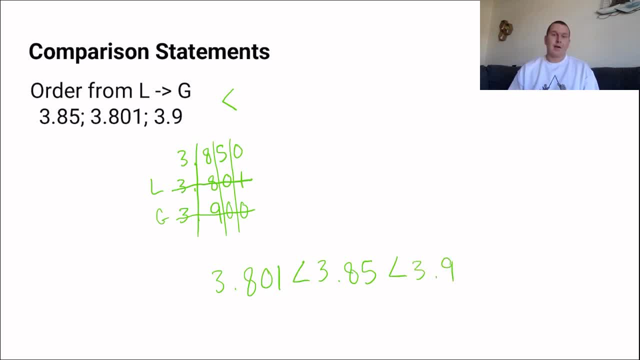 is less than 3 and 9 tenths. And to just ensure that we got the answer correct, we're going to read it out loud: So 3 and 801 thousandths is less than 3 and 85 hundredths is less than 3 and 9 tenths. 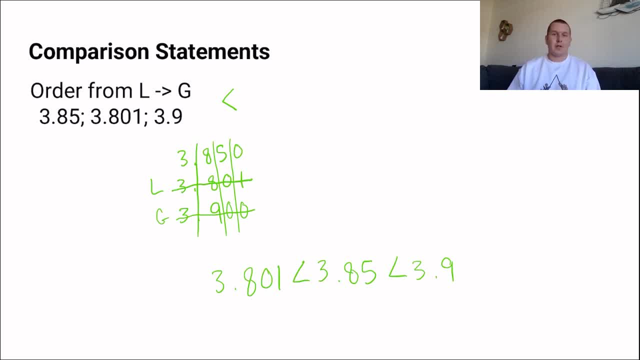 Notice, this time around I didn't include the zeros. I just wanted to show you that there's more than one way to do it. I personally like putting the zeros at the end, but you can do it this way as well. So it looks like we have a good comparison statement and we're ready to move on. 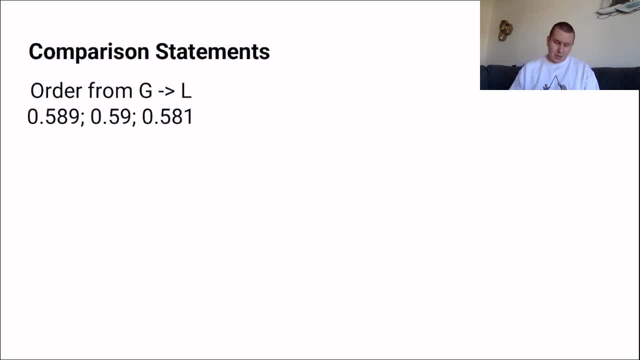 So we're going to start with that G, We're going to be using the greater than symbol. We're going to stack our numbers on top of each other Once again. there is no rhyme or reason between this. I always just go left to right. Don't start trying to order it from least to greatest. right now, Just not a. 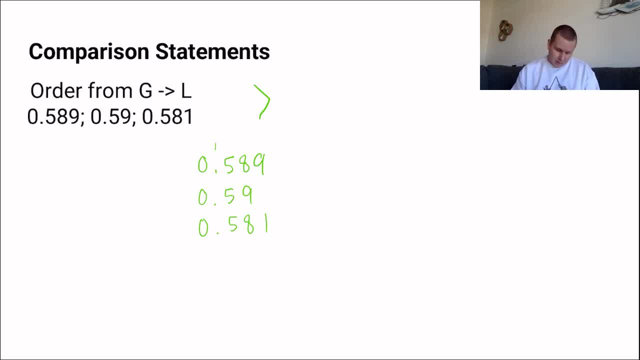 very good idea to guess why you're doing that. Then we're going to draw the lines in between. Helps us more easily compare. Add the zero to the end of that because it had a blank space, And now we're looking for the number that's the biggest. 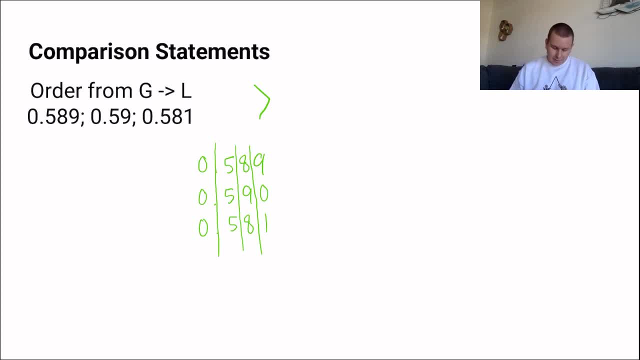 So in the one a place they're all zeros, tenths placed through all fives, but in the hundredths place our middle number has a number that's greater. So our comparison statement we'll start with this number and then we're going to use the greater than symbol. 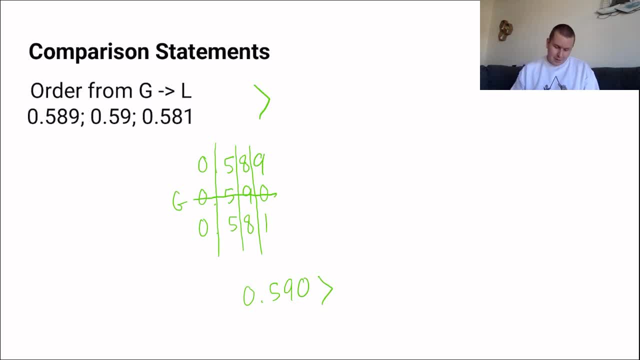 Now we're looking for the next biggest number. The next biggest number we'll have to go to the thousands place, And it looks like the nine is greater than the one. So 0 and five hundred eighty nine thousands will go in the middle, and then our final number would. 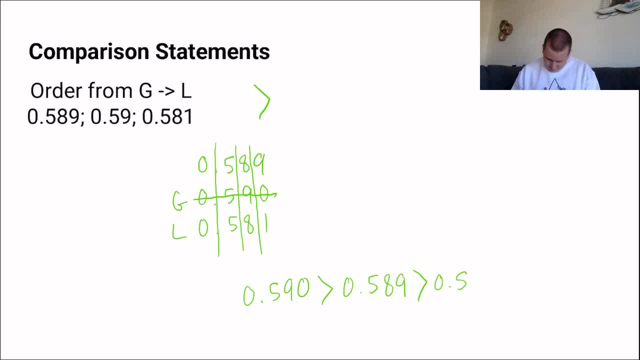 be this number and it'd be 0 and 581 thousandths. So just double check that we got it correct. We're going to read the comparison statement: 0 and 590 thousandths is less than 0 and 589 thousandths, which is less than 0 and 581 thousandths. I think I said the first number.